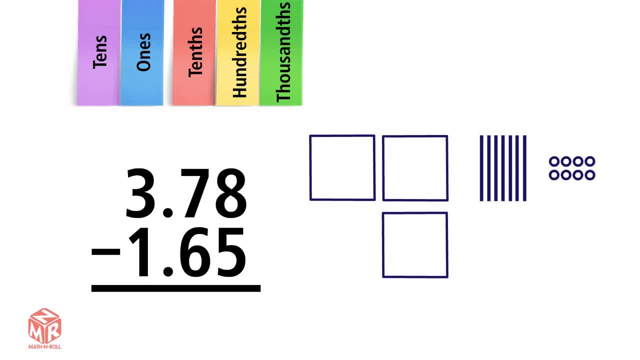 We represent the hundredths as circles. We subtract from right to left. so we start with the hundredths: 8 minus 5 equals 3, so we write that in the hundredths column. Let's do another example Next. we subtract the tenths: 7 minus 6 equals 1.. We bring down. 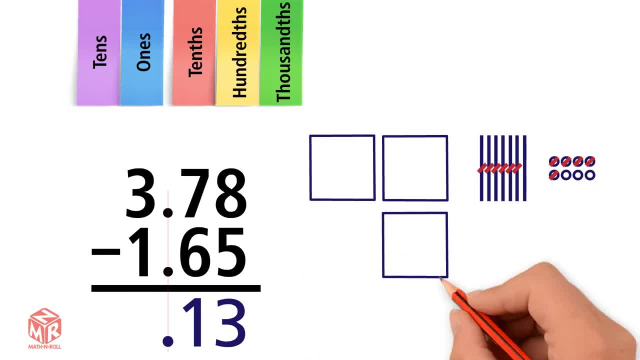 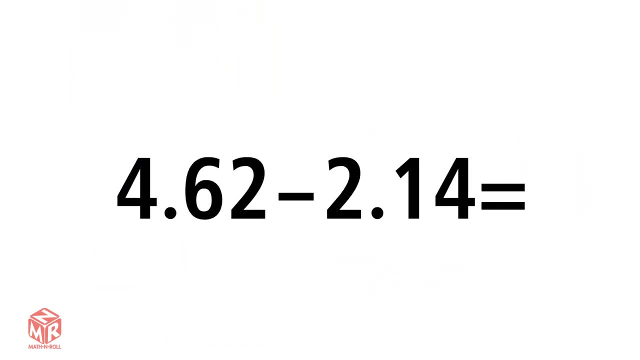 the decimal point. Now we subtract the ones: 3 minus 1 equals 2, so we write that in the ones column. So 3.78 minus 1.65 equals 2.13.. Let's do another example: 4.62 minus 2.45. 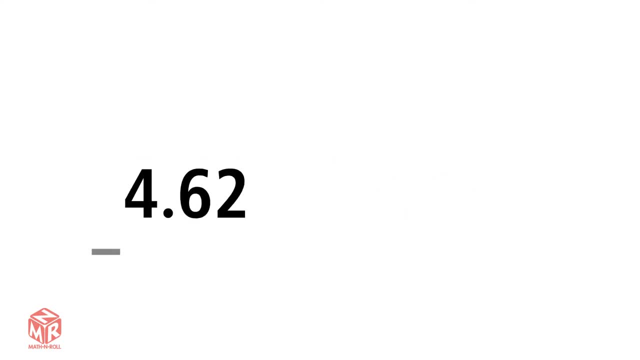 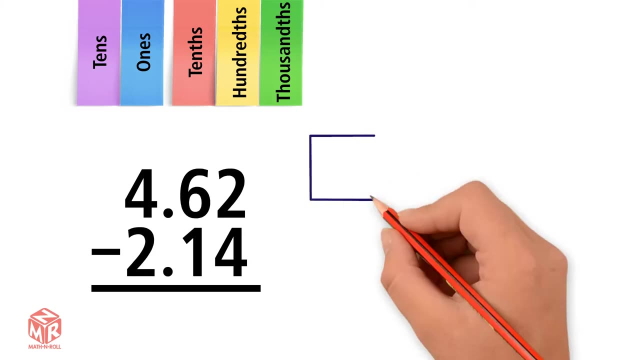 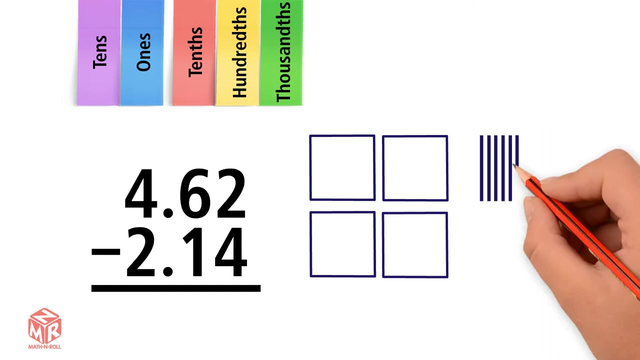 equals 2.14.. We start by lining up the decimal points. Let's draw 4.62.. 4.62 has four ones, six tenths and two hundredths. We subtract from right to left, so we start with the hundredths. 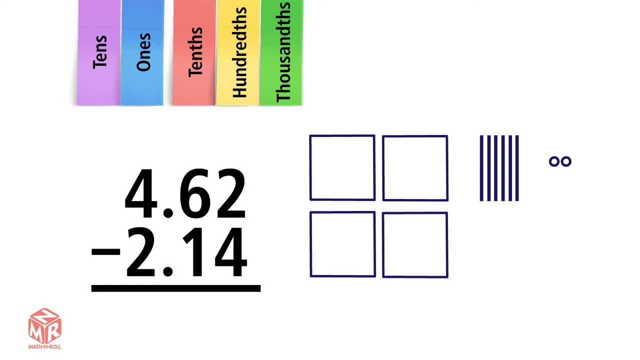 Are there enough hundredths to subtract 4 from 2? No, so we have to regroup. We regroup one tenth to make ten hundredths. Now we're left with five tenths and twelve hundredths. Subtract the hundredths 12 minus 4 equals 8, so we write 8 in the hundredths column. 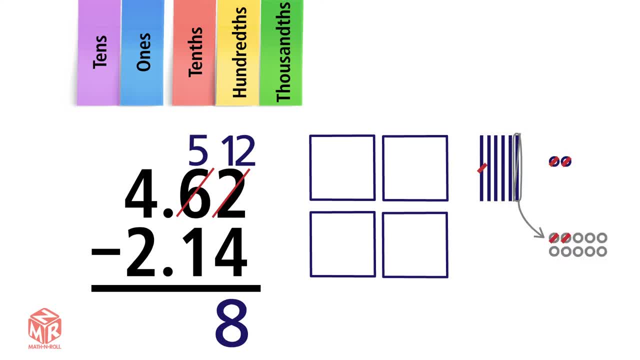 Now subtract the tenths, 5 minus 1 equals 4, so we write that in the tenths column and we bring down the decimal point. So in this example we have four plus one, which equals 1, so we subtract that 4 minus. 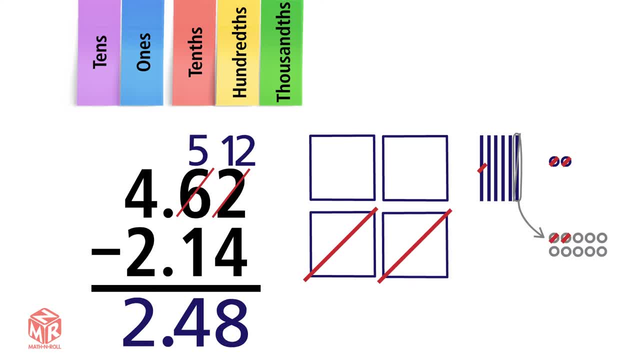 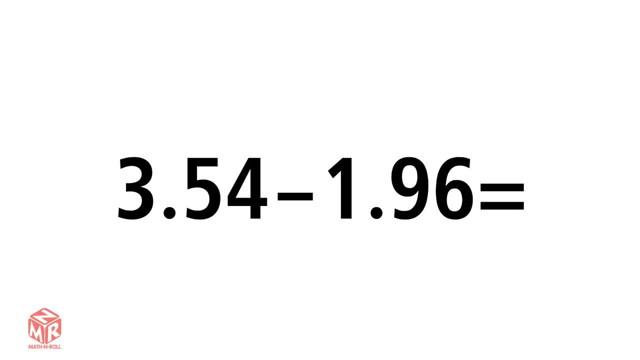 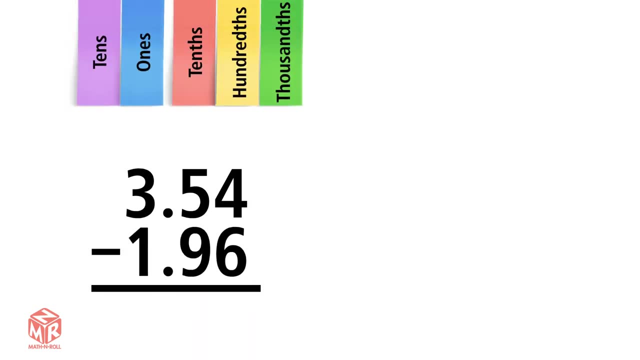 2 equals 2.. So the answer is 2.48.. Let's try another example: 3.54 minus 1.96.. We start by lining up the decimal points. Let's draw 3.54.. Are there enough hundredths to subtract? 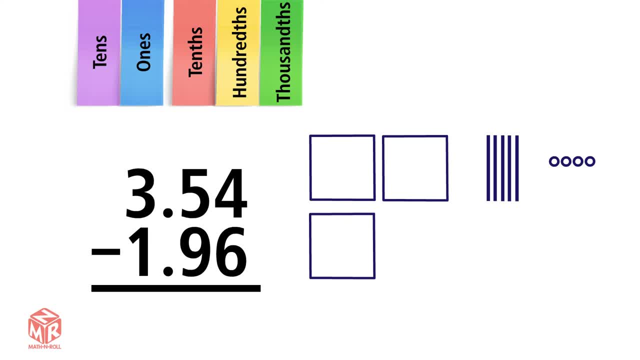 2? No, so we subtract 2.48.. hundredths to subtract 6 from 4? No, so we have to regroup. We regroup 1 tenth to make 10 hundredths. Now we're left with 4 tenths and 14 hundredths. Subtract the hundredths 14 minus 6 equals 8,. 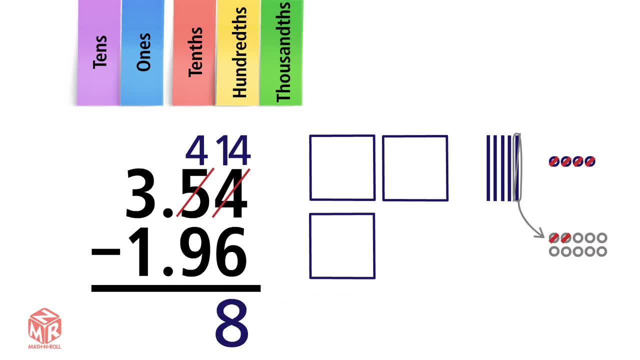 so we write an 8 in the hundredths column. Now we subtract the tenths. Can we subtract 9 from 4? No, so we have to regroup. We regroup 1 one to make 10 tenths. Now we have 2 ones and 14 tenths. Subtract the tenths, 14 minus 9 equals 5,. 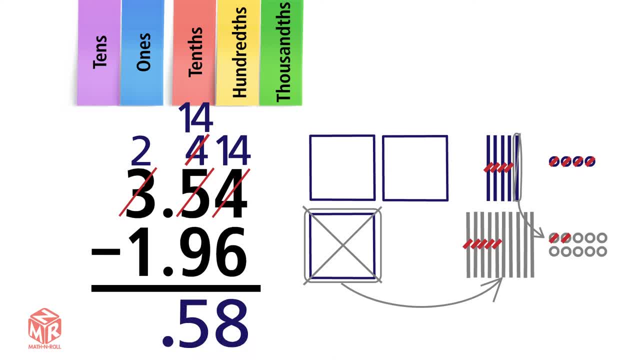 so we write a 5 in the tenths column and we bring down the decimal point. Now subtract the ones: 2 minus 1 equals 1, so the answer is 1.58.. Now let's do another example without modeling. 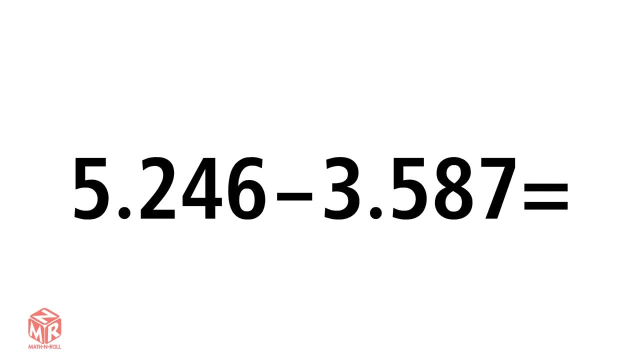 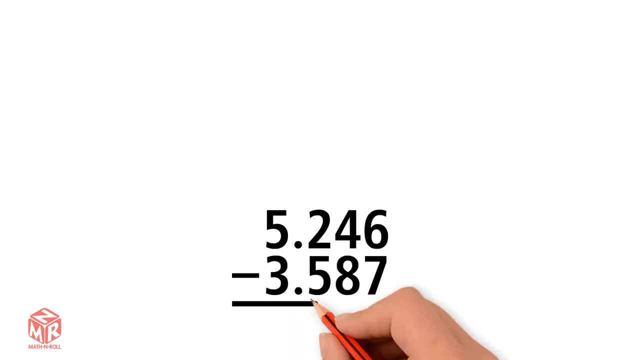 5 and 246 thousandths minus 3 and 587 thousandths. We start by lining up the decimal points. We start subtracting from right to left, so we start with the thousands. Are there enough thousands to subtract 7 from 6? No, so we regroup. 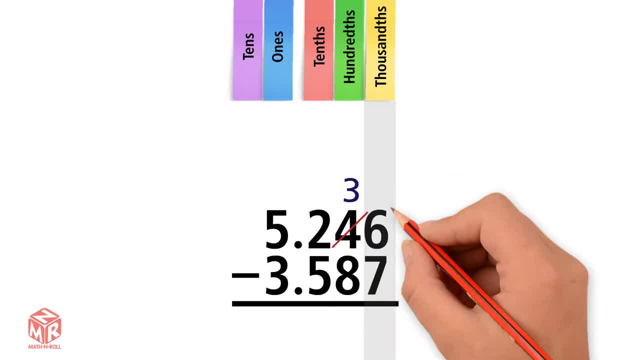 So we're left with 3 hundredths and 16 thousandths. Now subtract the thousands: 16 minus 7 equals 9.. Now subtract the hundredths. Can we subtract 8 from 3? No, so we regroup again. 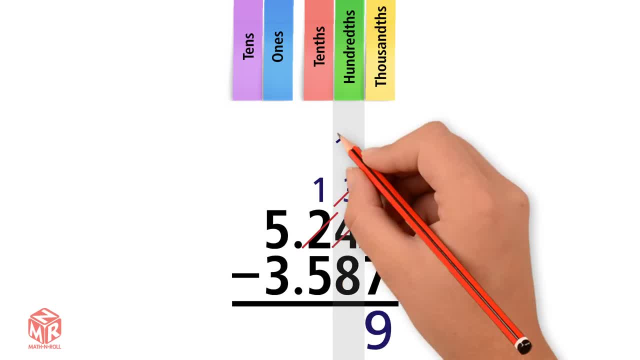 We're left with 1 tenth and 13 hundredths. Now we subtract the hundredths, 13 minus 8 equals 5.. So we write that in the hundredths column, Next subtract the tenths. Can we subtract 5 from 1? No, so we regroup again. We're left with 4 ones and 11 tenths. 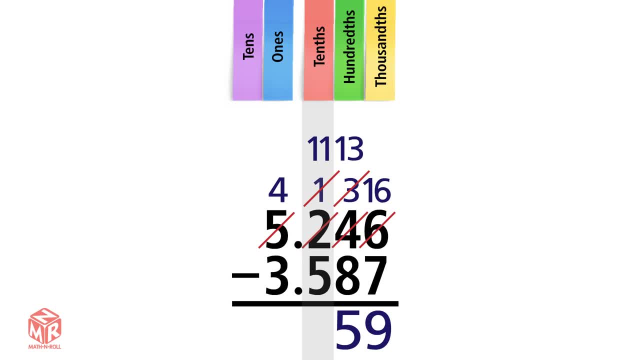 Subtract the tenths, 11 minus 5 equals 6, so we write 6 in the tenths column and we bring down the decimal point. Now, subtract the ones, 4 minus 3 equals 1.. So the answer is 1.58.. 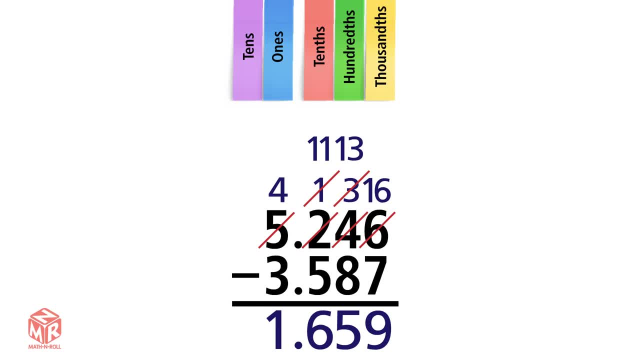 and 659 thousandths. If you thought this video was helpful, please leave a like. For more videos like this, please subscribe.